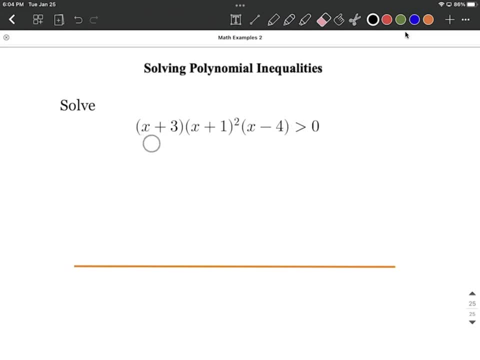 equal sign. I want to know, first of all, what values of x when you plug them in, because it's in factored form on the left-hand side. when I replace these x's with what number, would it make this factor equal zero? Same thing for each of these additional x's as we kind of move through. 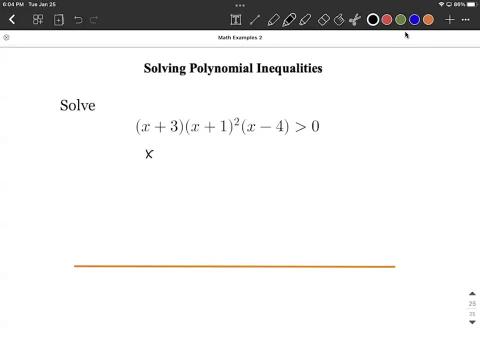 it. So the first thing I'm going to say is: well, it's going to be like when x equals negative three, when x equals negative one and when x equals positive four. I think if I plug in four minus four is going to make zero. therefore, the entire left-hand side equals zero. All right, next what? 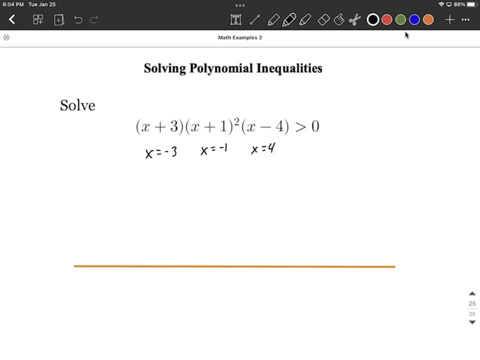 I'm going to do is place these values on the number line, So put them in number line order. So we have negative three, negative one and positive four. Now it's not to scale, but they are in the correct order on the. 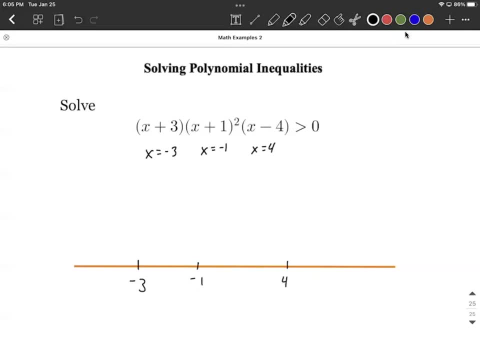 number line, and that's important. Okay, from here, what we want to do is test one value in between each section of this number line. So we split up the number line from negative infinity all the way to negative three, between negative three and negative one, etc. So we have four different. 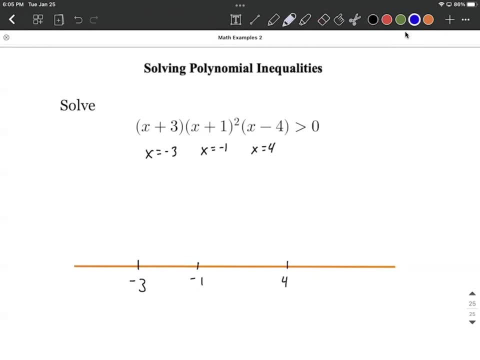 sections on this number line. So quickly we're going to move through and we're going to pick one value in each section. So anything to the left of negative, negative three, such as like negative four, And think about if we plug it in up into our 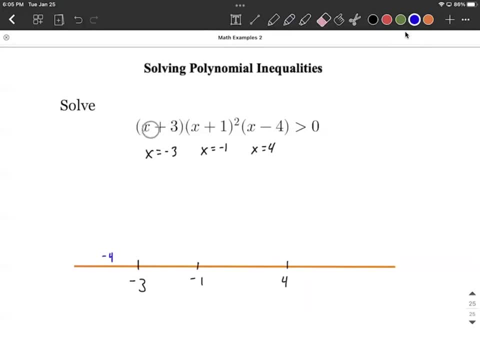 polynomial function. all we're going to care about is: does it turn out positive or negative for each factor? So as we plug it in, we have negative. four plus three makes negative one. All I'm going to do is say that's going to be a negative, though. Negative four plus three makes negative one. 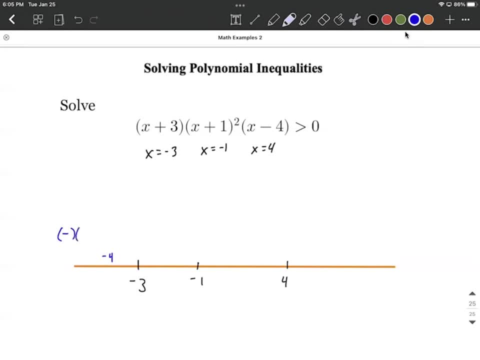 Overall, that part is negative and that's what's important. For the next factor we have negative four plus one, is negative three, but it's really going to be negative four plus three, So we're going to keep that in mind. So if we plug it in, we're going to have negative four plus three. 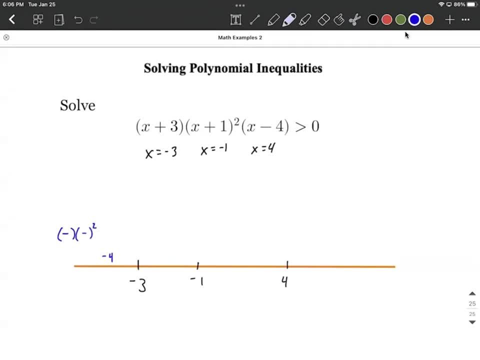 so we're going to have a negative four plus three. So we're going to have negative four plus three, And then negative four minus four more makes negative eight. But really, remember, we only care about negatives. Okay, from here let's count up how many negatives are being multiplied. 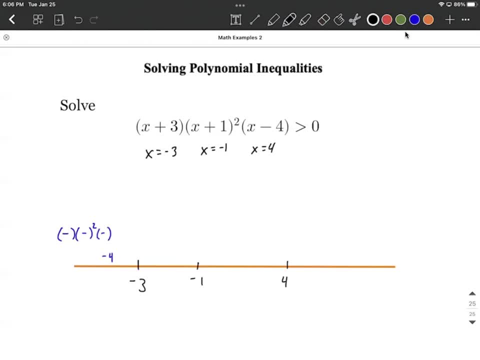 together over on the left-hand side. there You can see that we have one, two, because it's squared, that's going to be three and then a fourth one. So four negatives all multiply together to overall make it positive. So we're going to put a big positive up above our number line and that's. 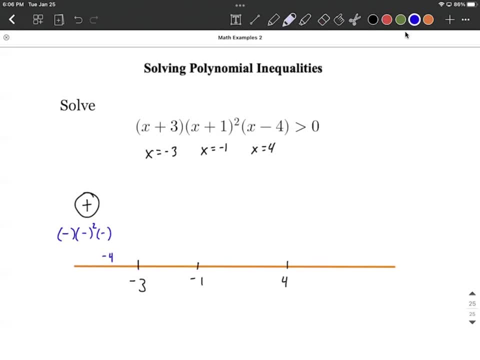 section. Next we're going to repeat it between negative three and negative one. Let's go with negative two And one at a time. we'll go negative two gets plugged in for each of the x's. So negative two plus three makes positive one. For that middle factor we say negative two plus one. 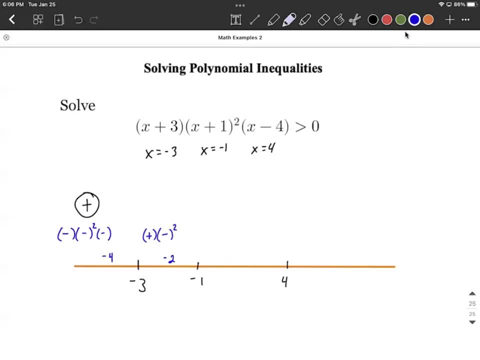 makes negative one, Then we're going to square it. So that counts as two negatives And then negative. two minus four makes negative six overall negative. So as you count these up, we had a positive and then three copies of negatives multiplied together. So the positive 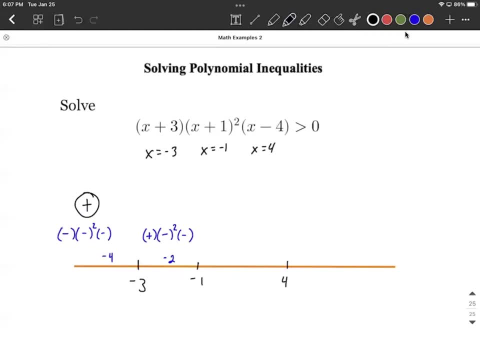 doesn't really affect positive or negative, but we have three negatives. An odd number is going to make negative overall in that section of the number line. Next, anything between negative one and positive four. we just repeat the process. I like plugging in zero because that makes life. 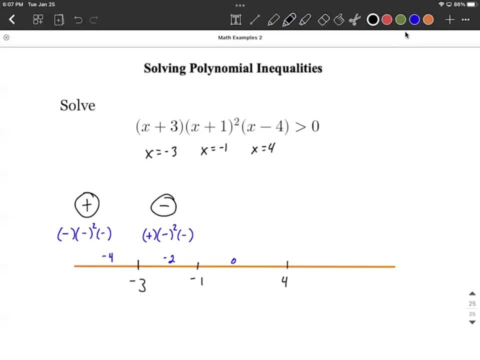 fairly easy as far as doing computations. So in for each of the x's we have: zero plus three makes positive. Zero plus one makes positive, Positive, it gets squared. And then zero minus four is a negative. So in this case we have three. 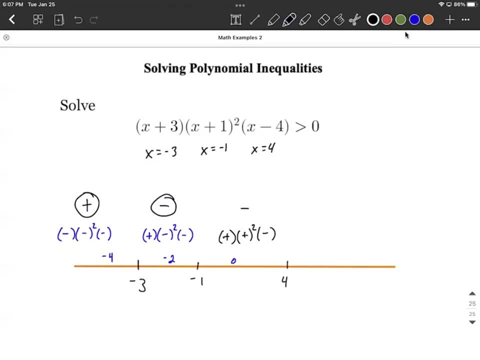 positives and one negative. Overall is going to be negative. One more on this number line We have anything to the right of four. So five, six, seven, eight, any of these values. I'm going to pick 10 because any of these values will return the same result. So plugging in a 10 for each of. 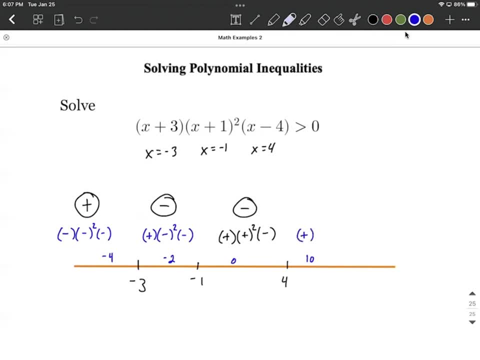 our x's we have: 10 plus three makes positive 13.. 1 makes positive 11, and then we square it and then 10 minus 4 makes positive 6.. So a bunch of positive values being multiplied together is overall going to give us a positive in that. 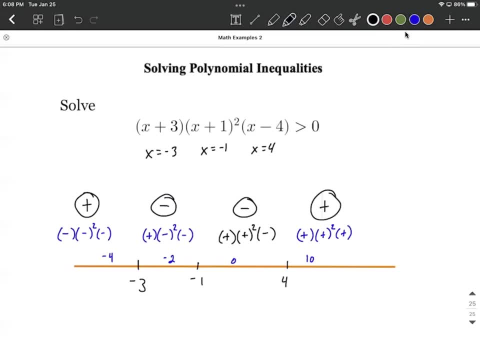 section of the number line. There was nothing special about me picking 10, except for it's in that section of the number line to the right of 4.. So each one of these values that we put below the number line, the negative 3, negative 1, and 4, those are when our actual function is going to. 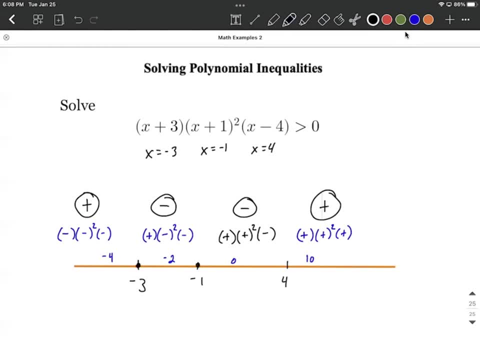 equal 0.. It's going to be on the x-axis. We're going to have a point on our x-axis for that polynomial function that's been factored on the left-hand side. But then the overall graph is going to be above the x-axis where we put pluses, positives, and then below the x-axis where we put 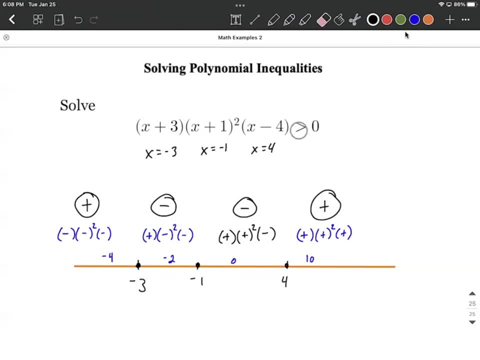 negatives. So now's the first time I've kind of referenced this inequality, sign being that it has to be greater than 0. So values that are going to be greater than 0, that means that it's going to be positive. So that's the first time I've kind of referenced this inequality, sign being that it has. 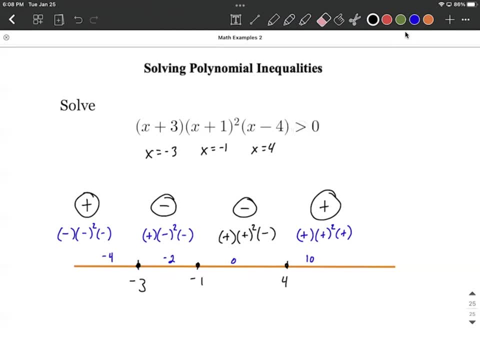 to be positive. Greater than 0 means positive. So for ours, what we're looking at is we're looking at the sections of the number line where it's positive over on the left-hand side and positive way over on the right-hand side, And then thinking about what kind of solution set or interval. 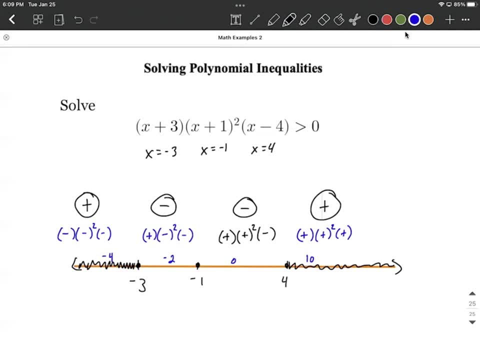 notation is going to go along with this. we'd say this one on the left-hand side goes from negative infinity all the way to negative 3.. Now, negative infinity is never going to be included, and negative 3 is also not going to be included in this situation, because this was a strict. 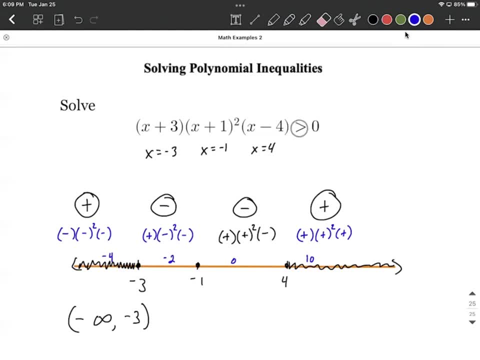 inequality of strictly greater than 0. It's not going to equal 0. We had another section of our number line that I shaded in where it was going to be positive over on the right-hand side. that goes from 4 off to the right-hand side forever. so 4 to infinity. Infinity is always going to get. 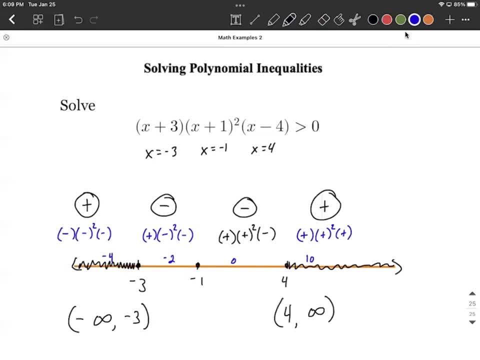 the open bracket, and 4 is also going to get the open bracket in this case as well. Again, because that's a strict inequality. if that's a strict inequality, it's going to be positive over on the left-hand side. So if we had a set of values that had been an or equal to, then we would include. 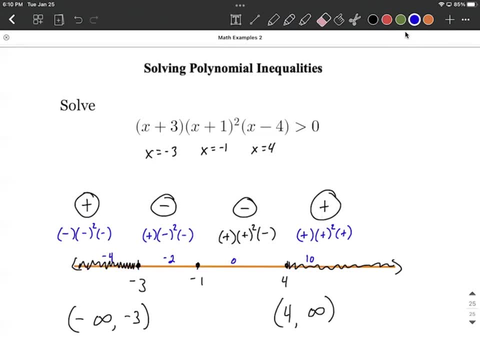 the endpoint. Now my solution set is correct in interval notation. here We may throw a union symbol in between for where we're looking for our positive values. As far as the graph goes, these endpoints at negative 3 and positive 4, if I were graphing this I would include: 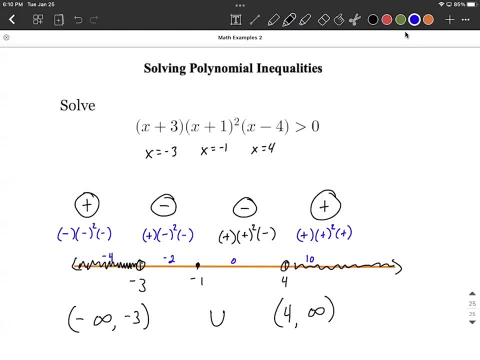 an open circle at each one of those values to indicate that that endpoint is not included. All right, now the alternate question we could be asked on this is: there's nothing special as we got going on this problem. that said, we were only looking for.